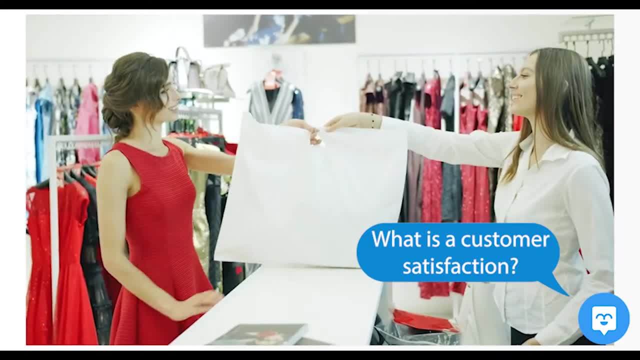 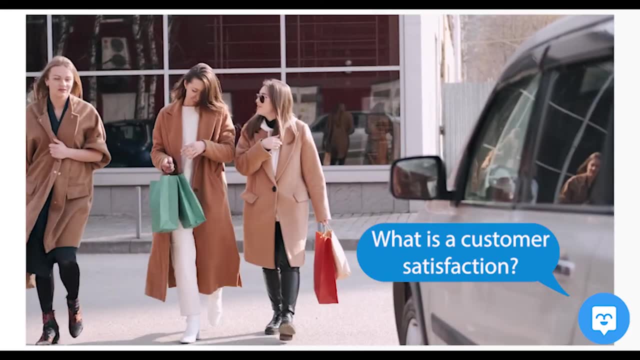 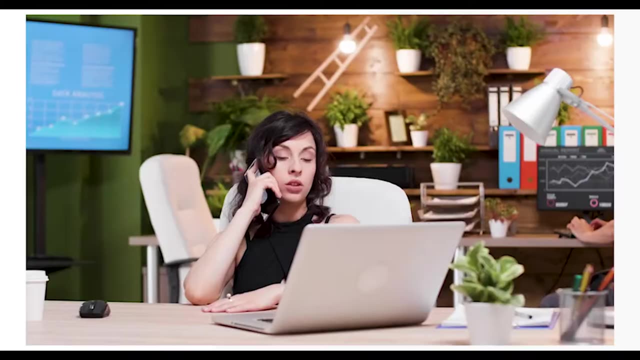 First, what is customer satisfaction? In the most simple definition, customer satisfaction is a metric that refers to the degree to which the customer expectations have been met. Meet your customer expectations and your customers will be satisfied. Exceed their expectations and they'll be delighted. You could also miss the mark when meeting customer expectations. 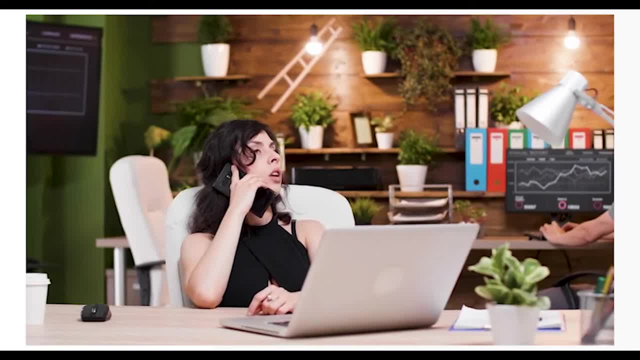 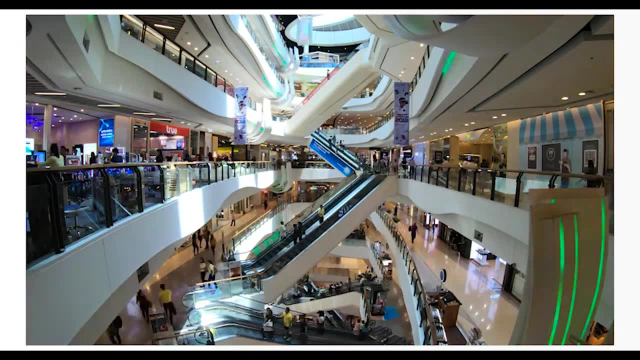 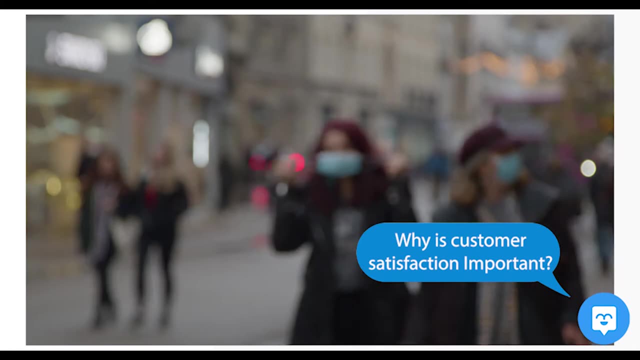 resulting in low customer satisfaction scores and displeased customers. Both scenarios can end up having a significant impact on your business, even financially. Why Customer Satisfaction is Important. The impacts of customer satisfaction on your business can be both significant and lasting, especially when you consider the 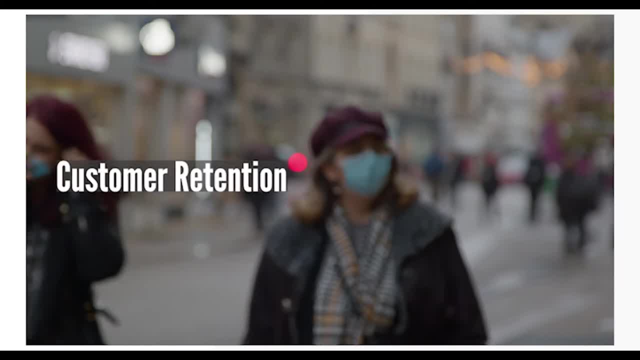 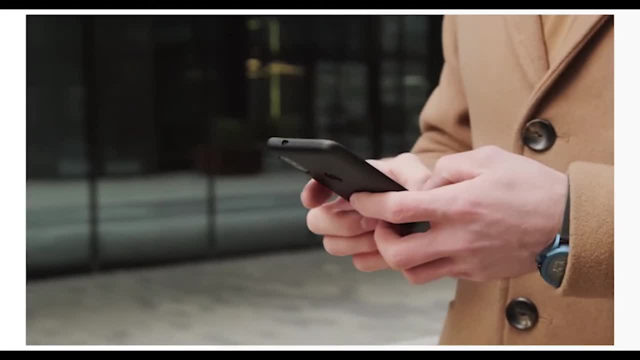 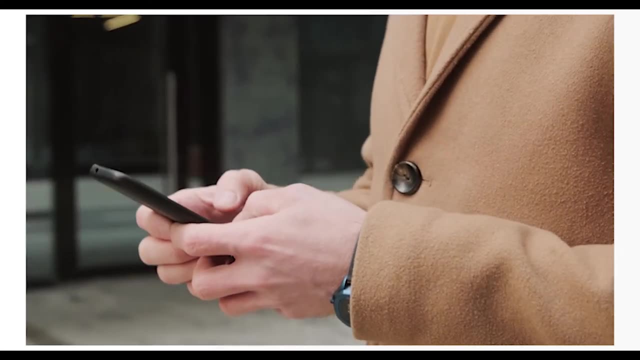 effects that customer satisfaction scores have on customer retention and loyalty. Satisfied customers are more likely to stay as one of your customers and are more likely to advocate for your business. They are also more likely to post positive reviews and testimonials of your business online and on social media. Customer satisfaction can end up affecting your bottom. line. With higher customer retention also comes higher customer revenue, as it's generally cheaper to retain a customer than to acquire new ones, And with more positive reviews and loud advocates for your brands, your acquisition costs can also be reduced. On the other hand, 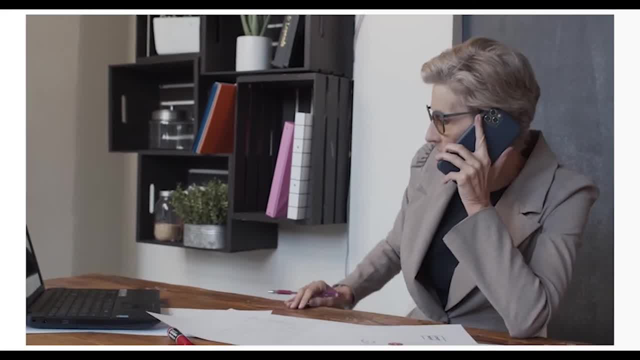 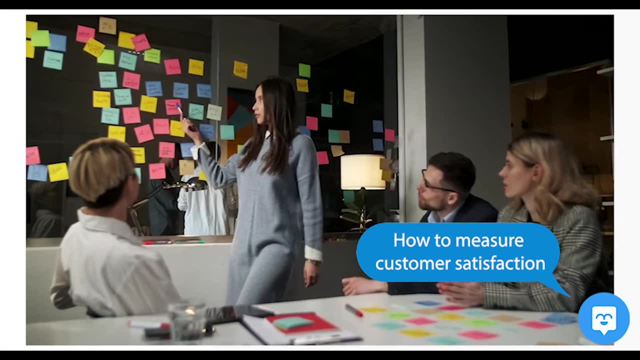 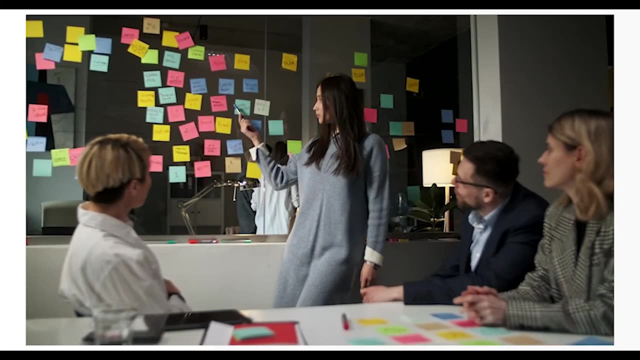 low customer satisfaction can result in low customer retention, negative reviews and a negative brand image. How to Measure Customer Satisfaction? Customer satisfaction can be measured in many different ways, the most common being the customer satisfaction score or the CSAT score. CSAT is the 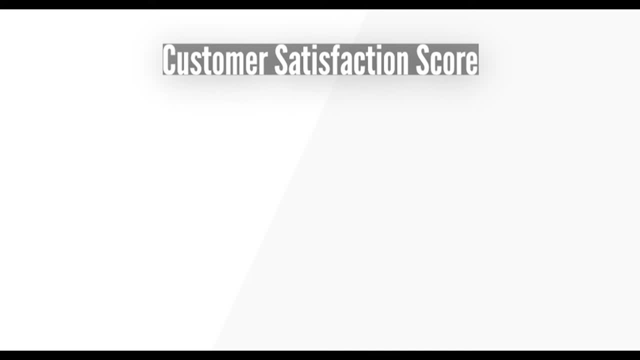 average score that your customers are likely to get in order to find your overall CSAT score. CSAT is the average score that your customers are likely to get in order to find your overall CSAT score. After collecting all the responses, the average scores are calculated in order to find. 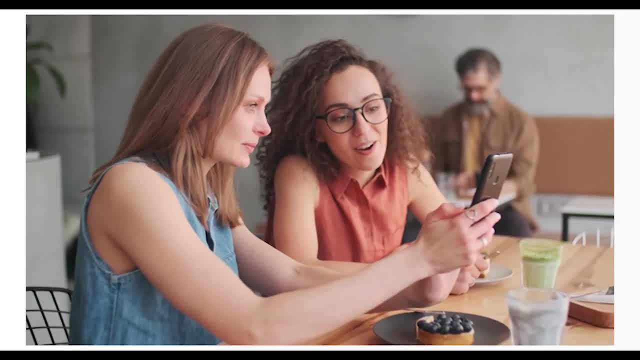 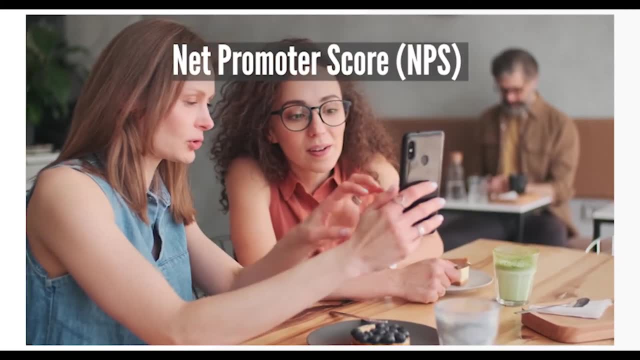 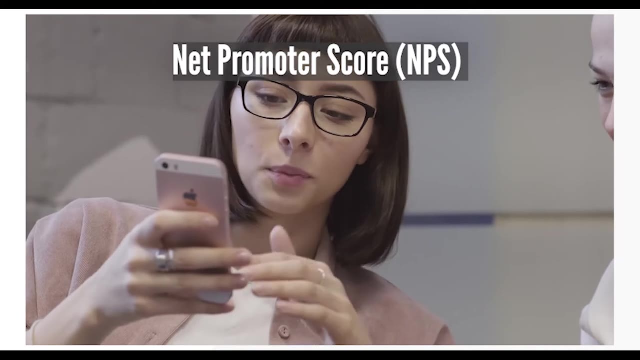 your overall CSAT score. Another popular metric used to get a sense of your customer satisfaction is the Net Promoter Score, or NPS. NPS measures how likely your customers are to recommend your business to others, based on their experience. This score is calculated in asking customers. 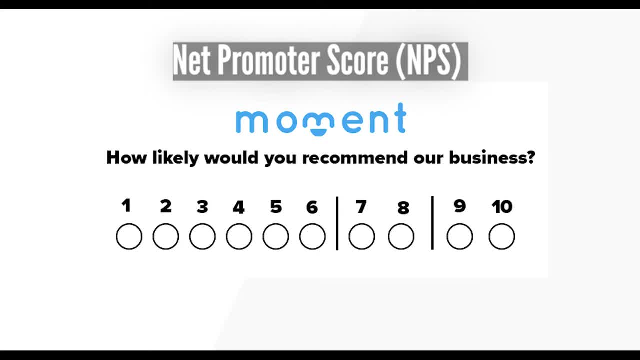 how likely they are to recommend your business to a friend or colleague in a scale of 1 to 10.. Customers are then categorized based on their answers: Promoters answer between 9 to 10 and passives answer between 7 to 8.. Detractors answer 6 and lower.